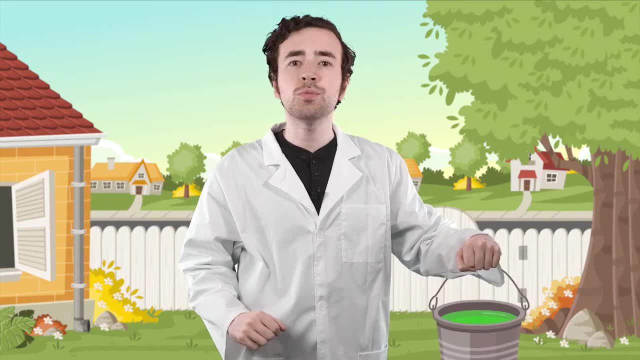 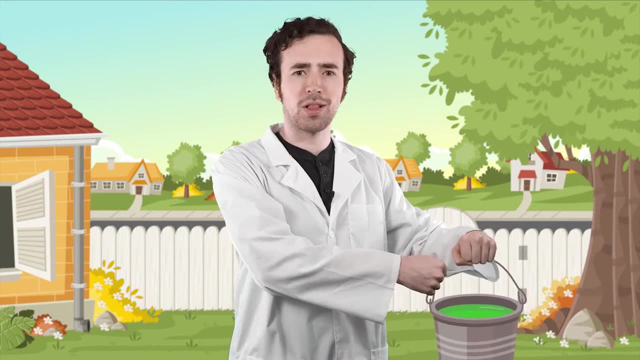 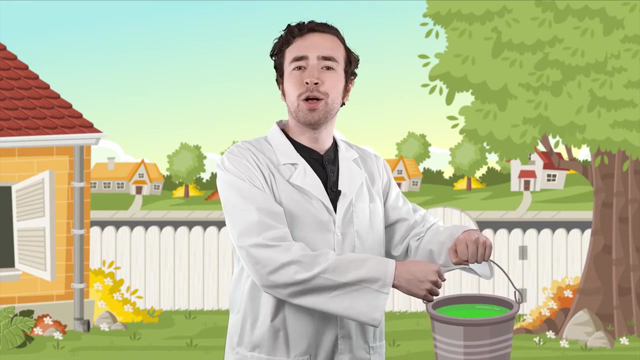 slime over to my parents' house and then up the stairs into my sister's room. I don't know if you noticed, but I've been at this all afternoon and I just can't move this bucket. I think it's time to enlist the help of some simple machines By the end of today's lesson. 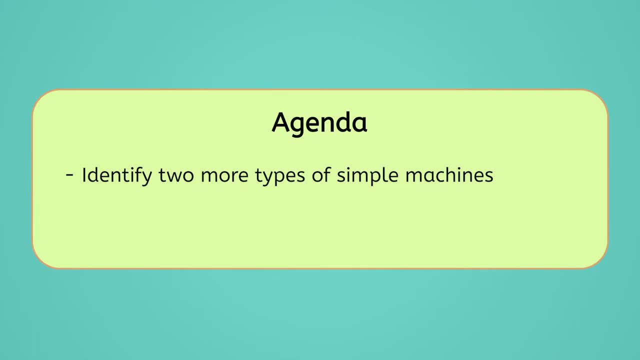 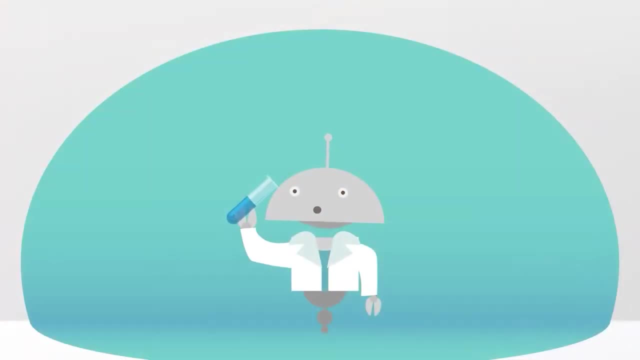 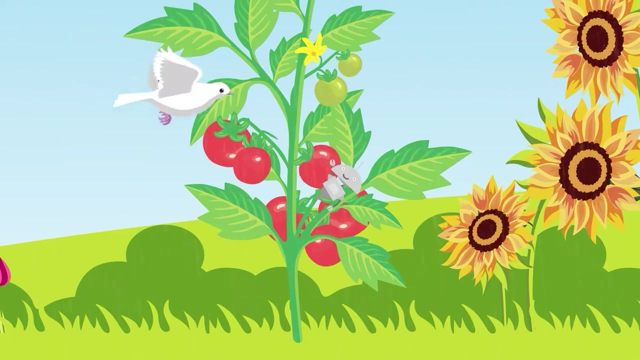 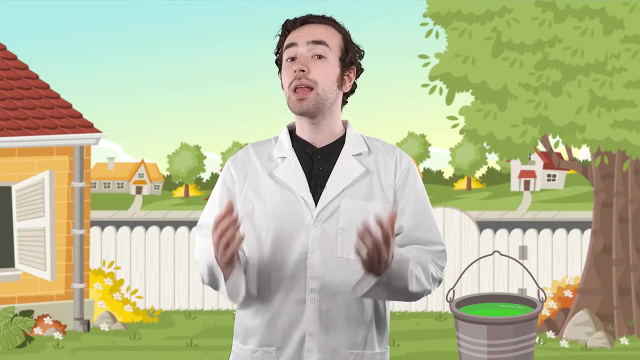 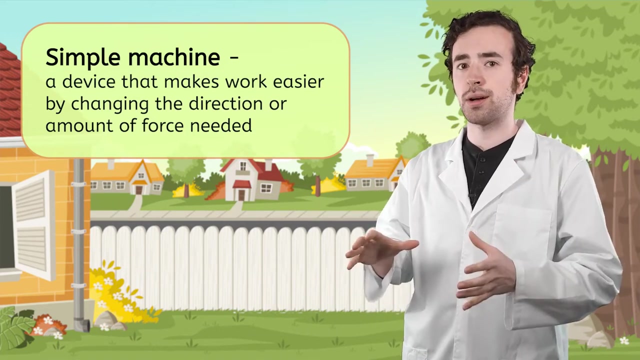 you will be able to identify two more types of simple machines and explain how they help us to do work. Let's get into it So. in our last lesson we learned that simple machines are devices that make work or exerting force on objects to move them easier, either by changing the direction or the 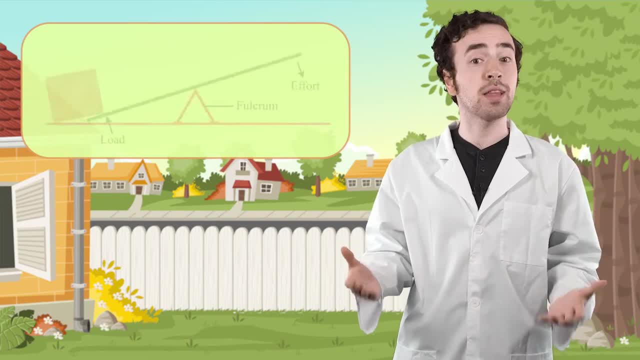 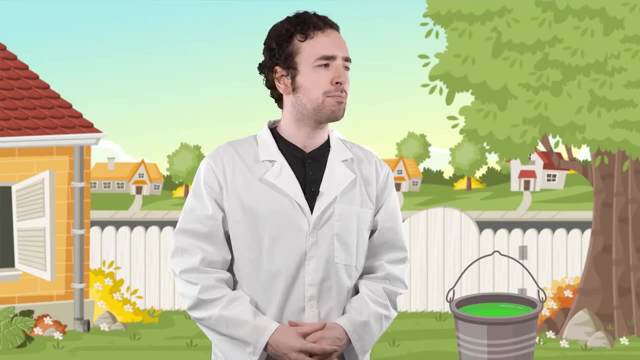 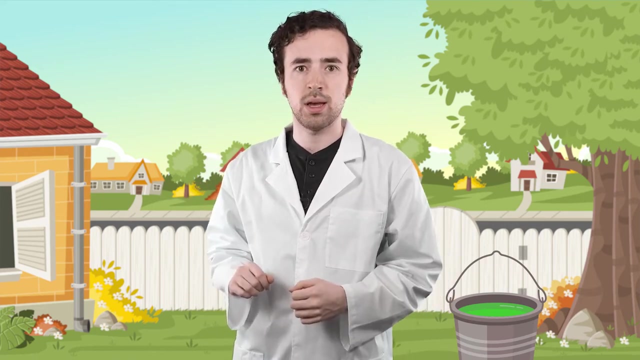 amount of force required. We also learned that levers are very helpful, simple machines that we can use to lift heavy objects. Trouble is, I don't really need to lift my bucket, I just need to move it down the street to my parents' house. Luckily, I think I know a simple machine that. 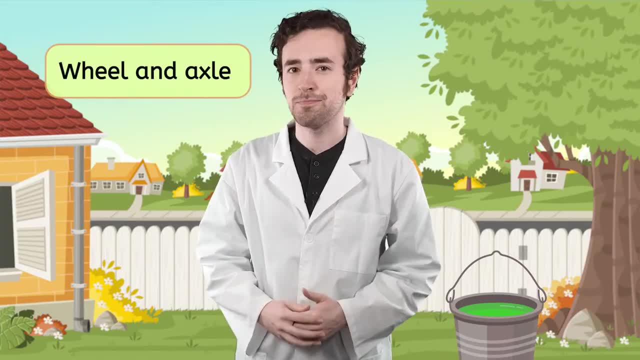 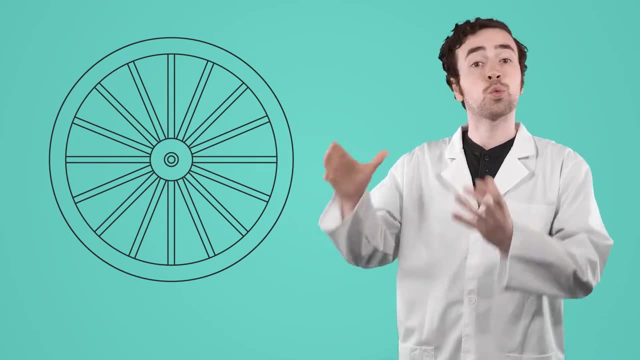 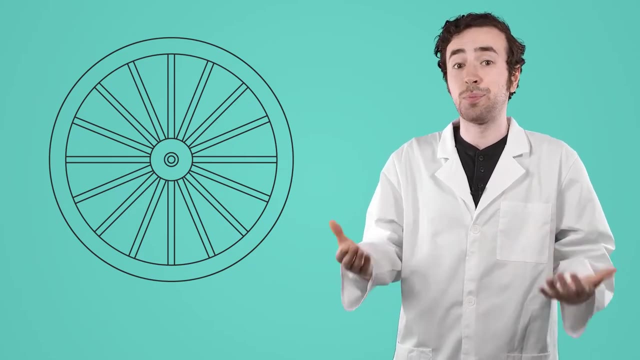 will do the trick: The wheel and axle. You've probably heard of a wheel before. It's a round, disc-like object that can roll on its side By itself, though a wheel actually doesn't do that much to help us make work easier. 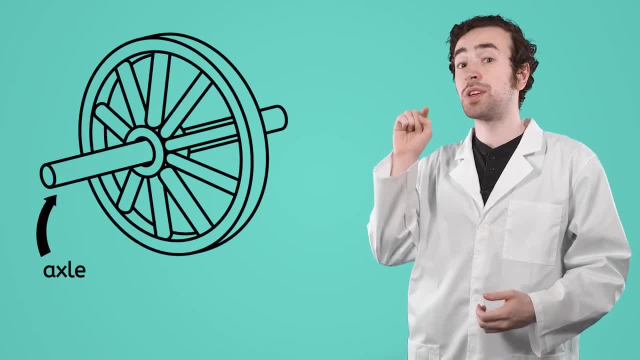 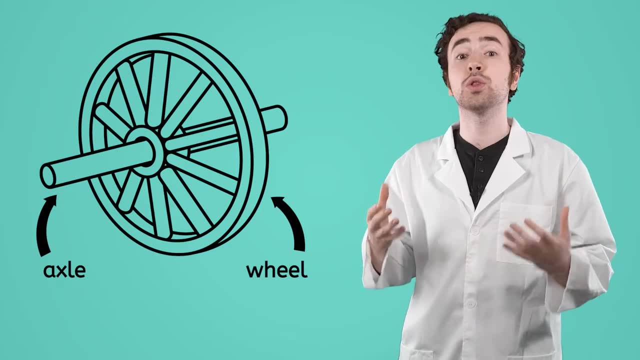 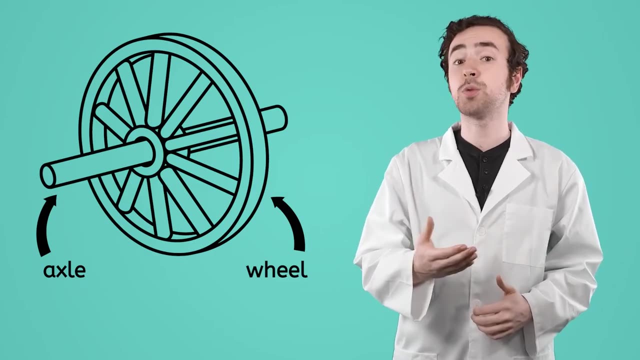 But once you put an axle or a rod through the center of that wheel, then the possibilities are endless. Axles are what allow us to carry loads on top of the wheel And they allow us to connect several wheels together. Axles can also be what causes the. 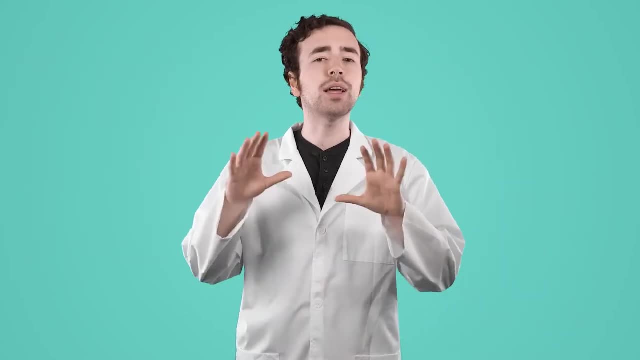 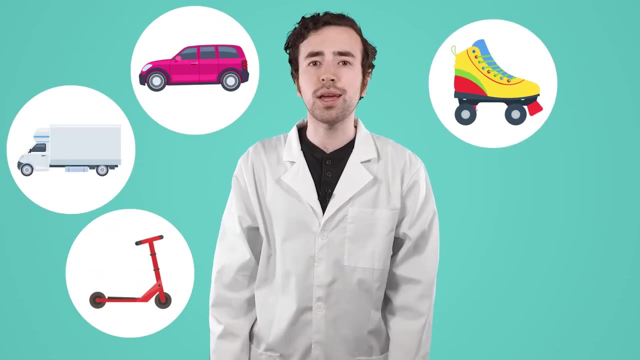 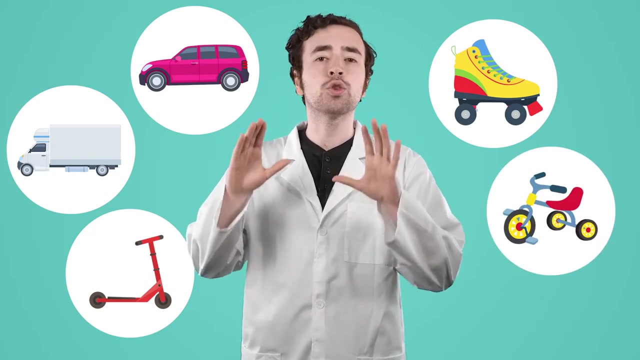 wheel to turn in the first place. Objects that use wheels and axles are everywhere: Cars, trucks, scooters, roller skates, even my little sister's tricycle- all use wheels and axles. They are a crucial part of being able to carry heavy loads over long distances, So let's get into it. 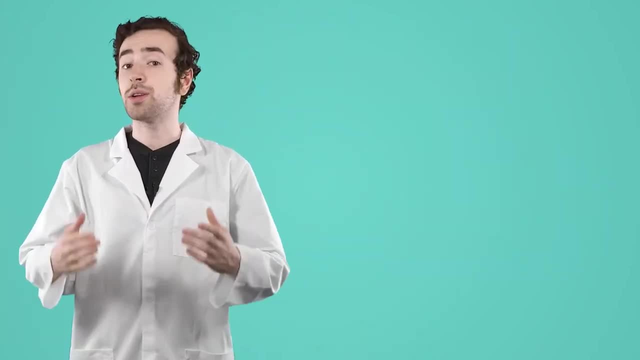 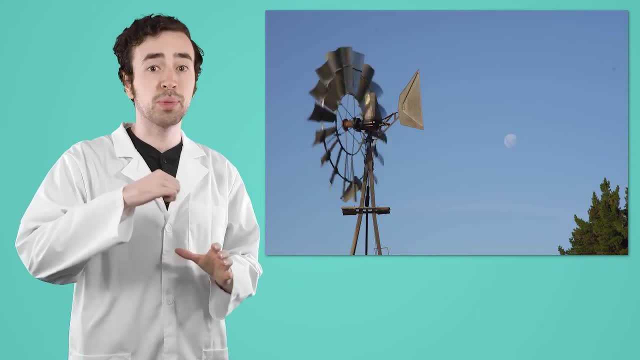 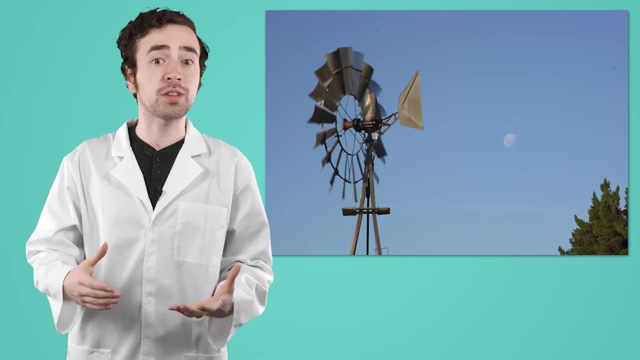 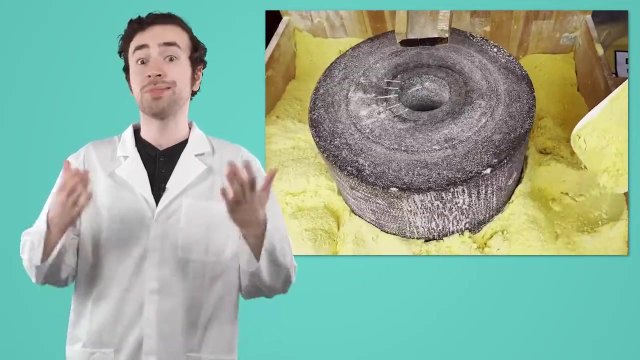 for example, The wind pushes on the blades which are connected to a wheel, And that wheel spins an axle. Now that redirected force can be used to accomplish tasks like grinding wheat to turn into flour or even generating electricity. Even a doorknob is an example of a 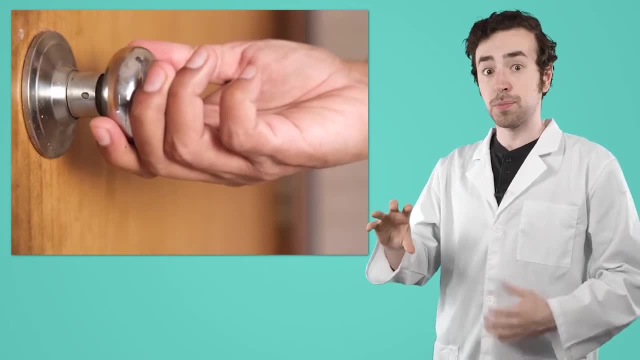 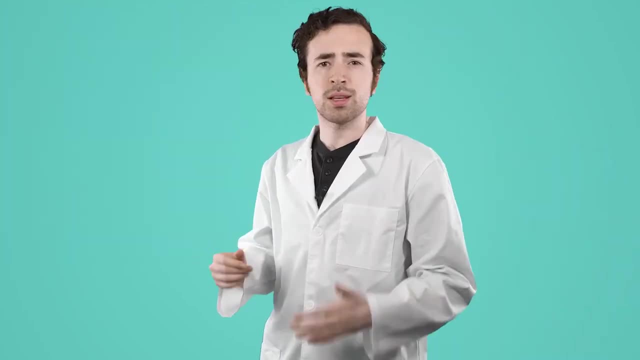 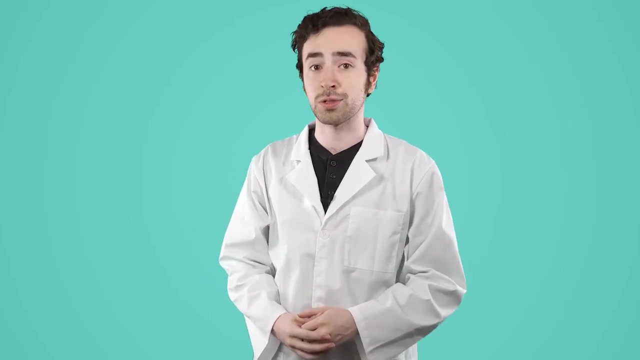 wheel and axle at work. Spinning the knob, the wheel turns an axle which releases a latch allowing the door to open. Can you think of any other places where wheels and axles are used? Pause the video now to jot down your thoughts in your guided notes. 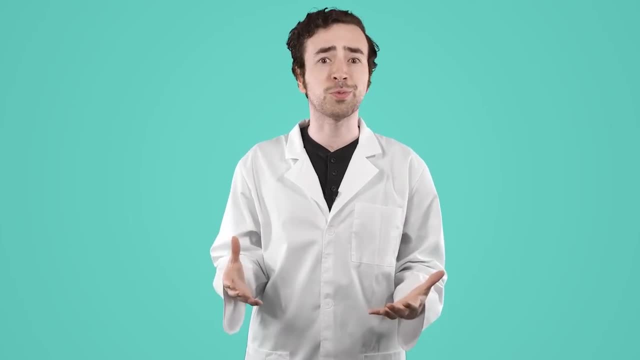 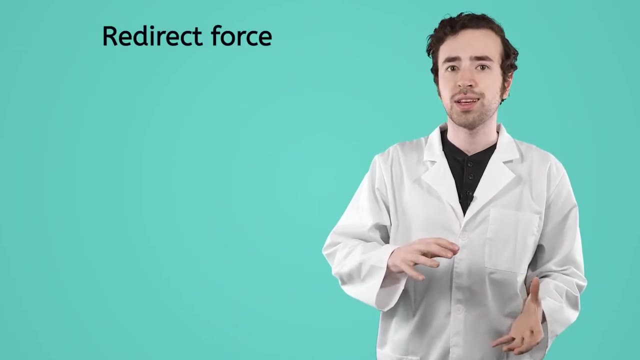 Wheels and axles are probably so common because we use them for all sorts of different things. Sometimes we use wheels and axles to work for a company, sometimes we don't. So for this episode, wheels and axles to redirect force, sending it in directions that would be hard for us to do. 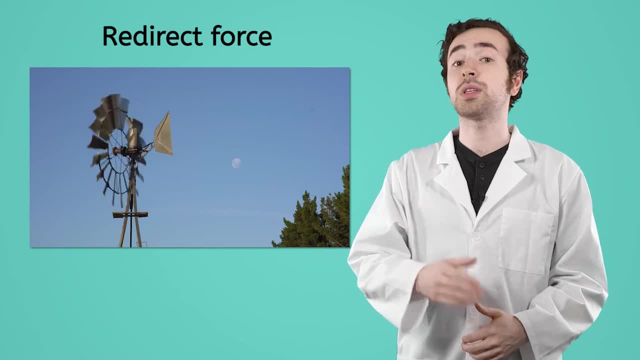 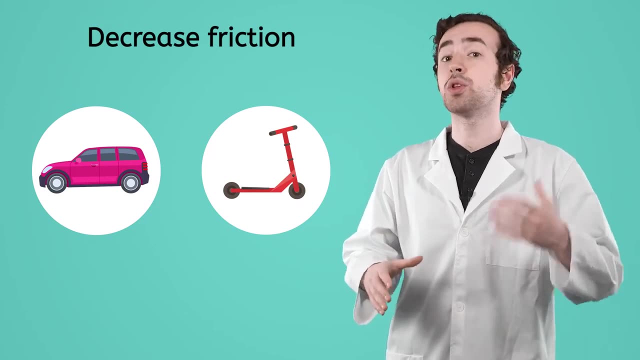 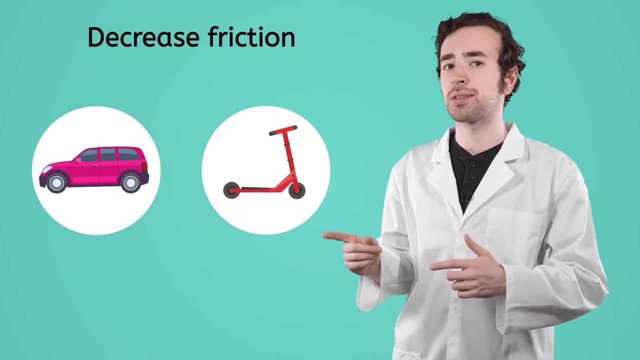 ourselves, like with the windmill. When wheels and axles are used in transportation, like in cars and scooters, they actually decrease the amount of friction between the load and the ground. Less friction means less force required to move the object over a long distance. 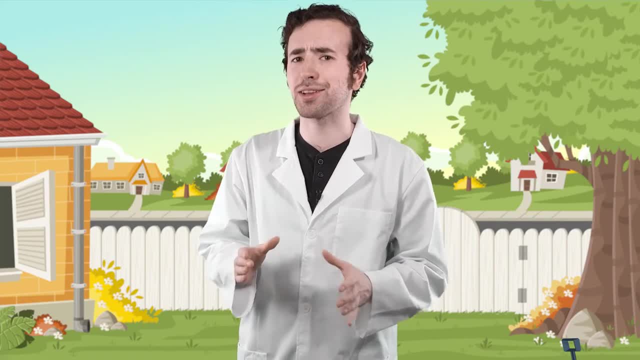 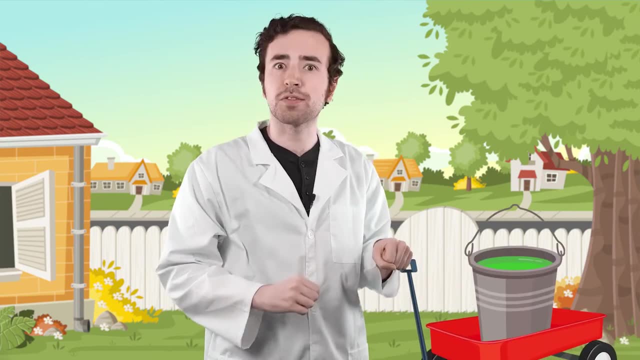 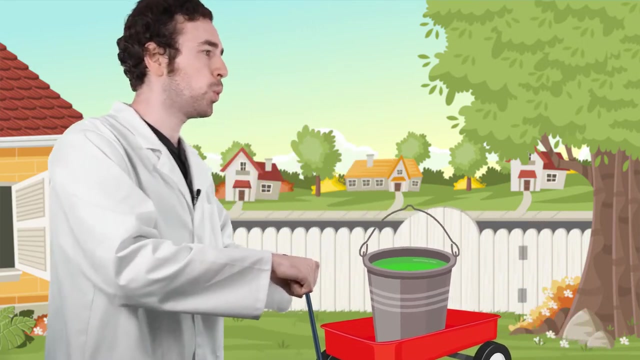 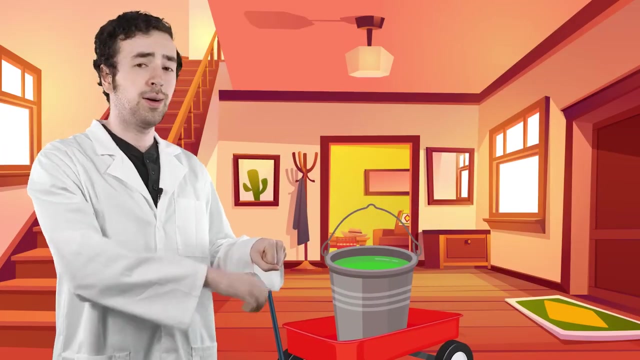 That actually sounds like exactly what I need right now. My wagon has wheels and axles at the bottom. If I put my bucket of slime into that, that'll make it much easier to get the bucket home. Let's go All right, mission accomplished, Only now we have to get the slime. 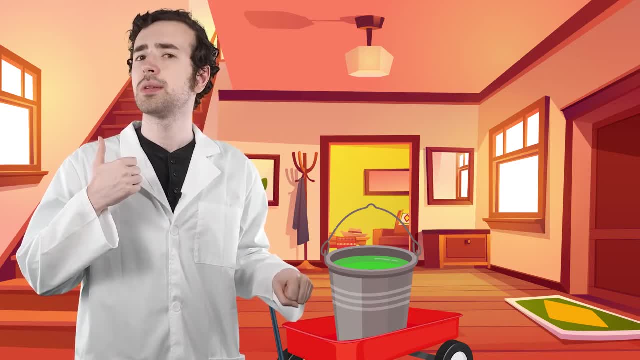 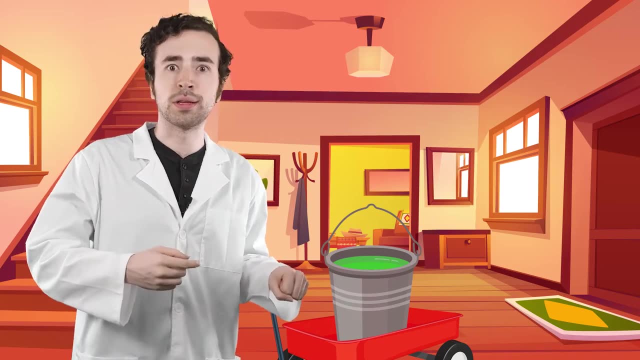 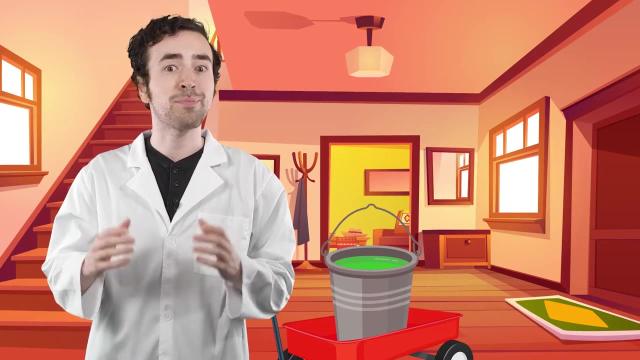 up the stairs to my sister's room. Wheels and axles are great, but I don't think my wagon is going to help me safely get all this slime up a flight of stairs, So maybe a different simple machine can help us out here- A pulley. A pulley is another simple machine that also uses a wheel. 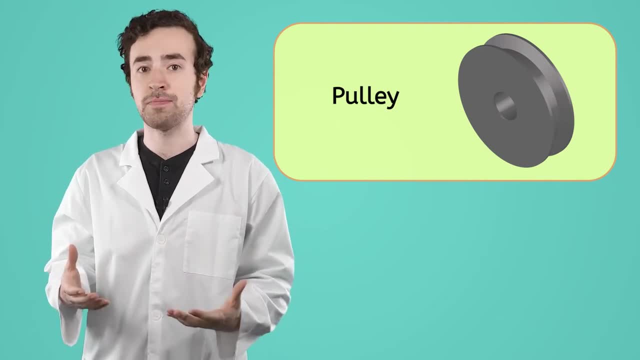 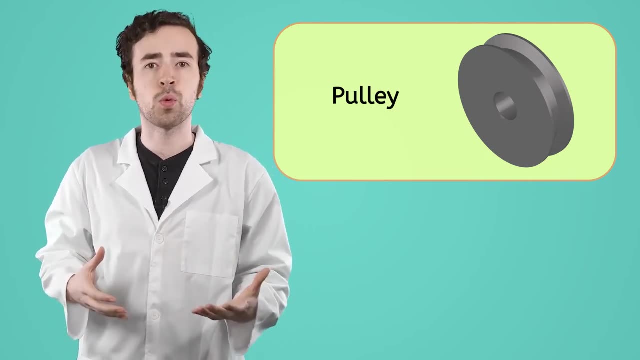 only in a much different way than with a wheel and axle. This wheel has a special groove around the wheel, So it's going to help us get the slime up the stairs to my sister's room. its edge that's designed to hold a rope or some chains If we want to lift an object using a 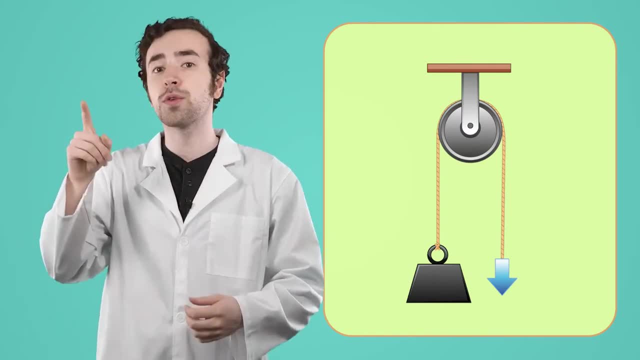 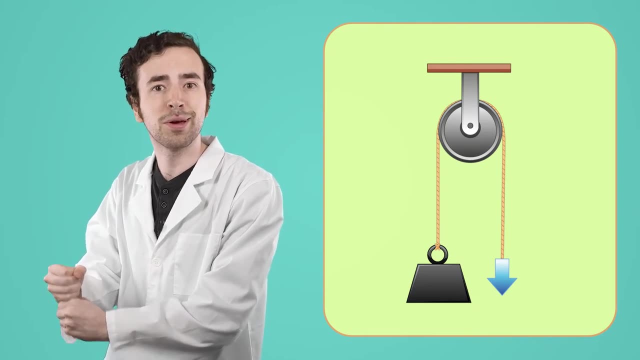 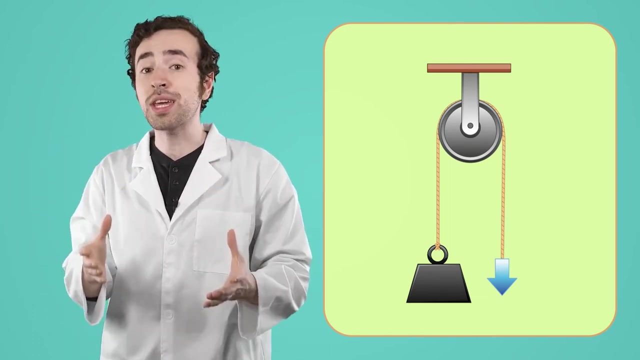 pulley. we can tie a rope to it, put the rope over the wheel and then just pull the rope down from the other side to lift the object. Get it, Pull Pullee Pulleys are great at redirecting force. 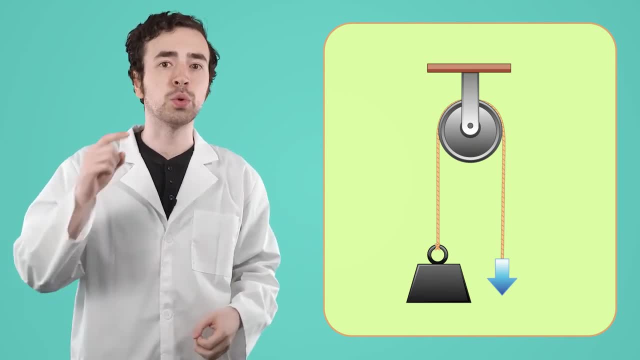 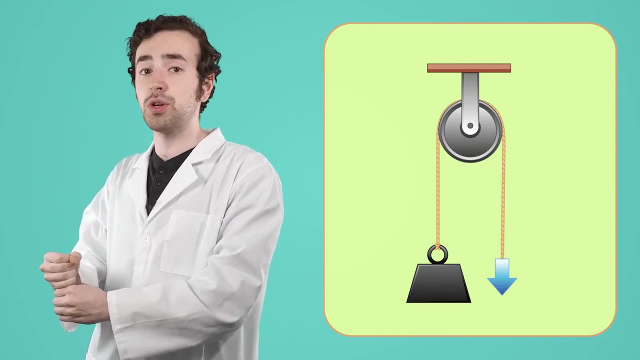 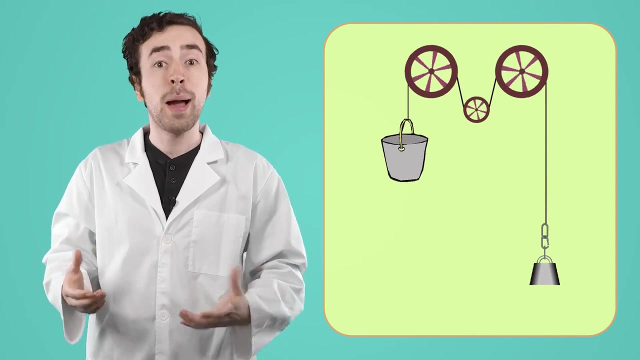 Even though it will take the same amount of force to lift this object with a pulley. pulling down on something is usually a lot easier for people to do than lifting an object up themselves. We can even decrease the amount of force required by adding more wheels to the pulley. Pulleys are 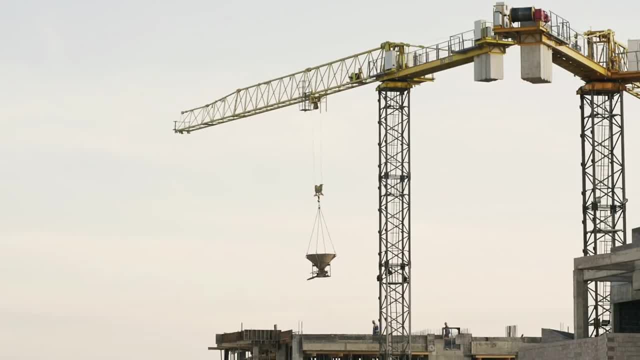 everywhere. If you've ever seen a big construction site, you've definitely seen a crane which is basically just a small crane. If you've ever seen a big construction site, you've definitely seen a crane which is basically just a small crane, which is basically just a small crane. If you've ever 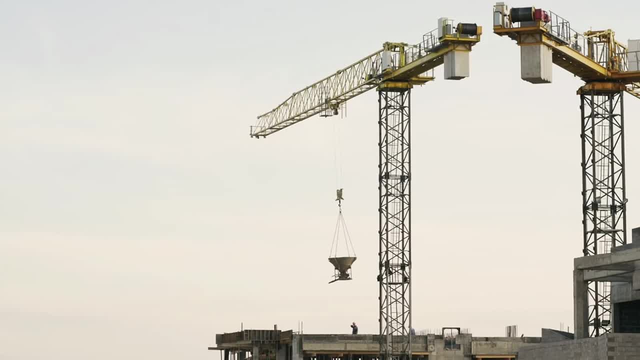 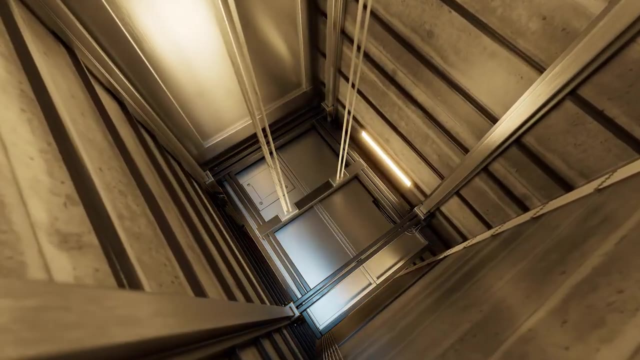 just a big pulley. Cranes are used for moving heavy materials and other machines between the top and bottom of buildings. They're super important to construction And once the structure is built, pulleys are used inside of it too. The elevators used to lift and lower people between floors. 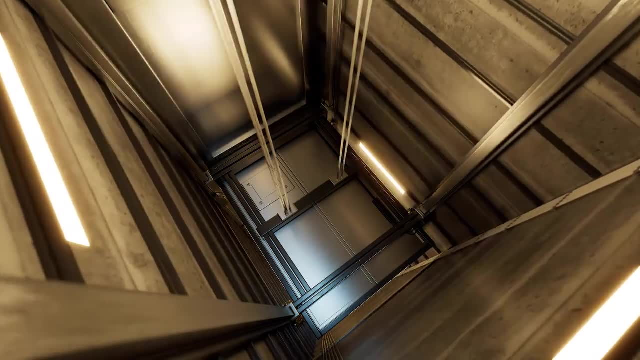 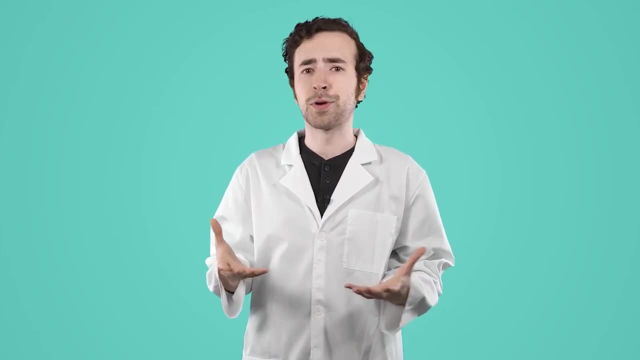 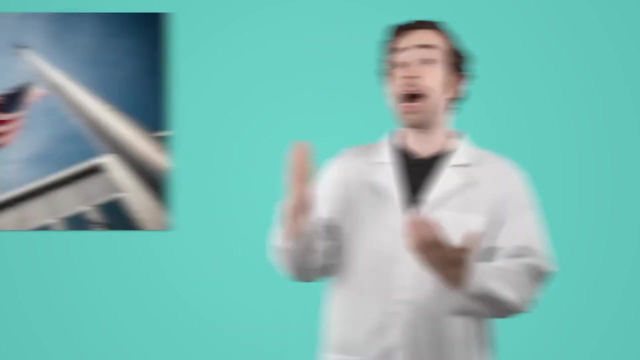 operate using a pulley system to move the elevator cars up and down. Pulleys are great for helping us lift heavy loads, but they're also just really good at helping us get objects to inconvenient spots that are hard for us to get to, like the top of a flagpole or even the top of your window. 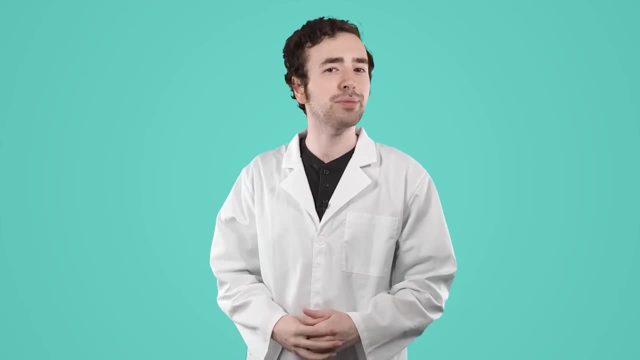 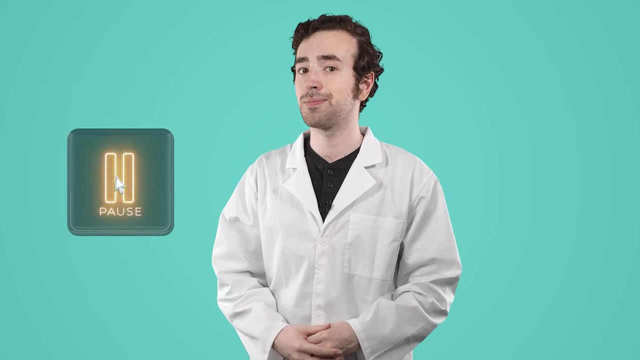 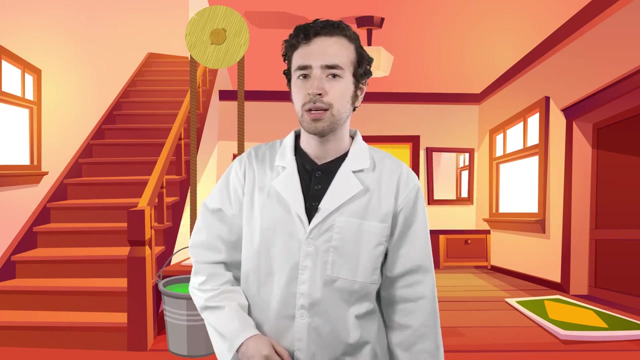 Can you think of any other places where you've seen pulleys in action? Pause the video here to write down your observations in your guided notes. I think a pulley is the perfect, simple machine to get my slime to the top of the stairs. 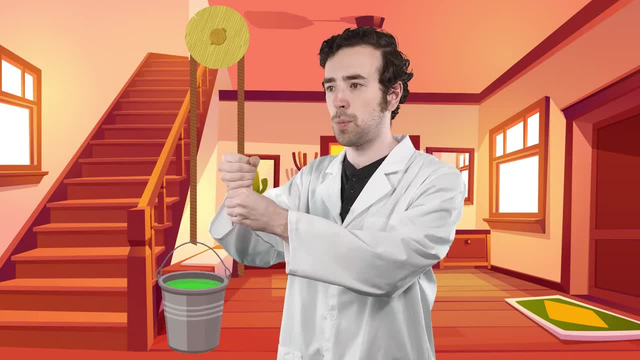 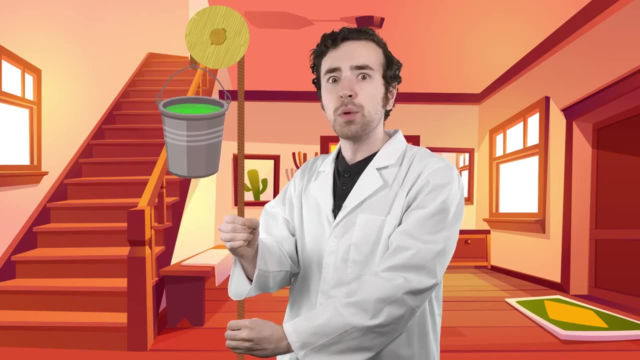 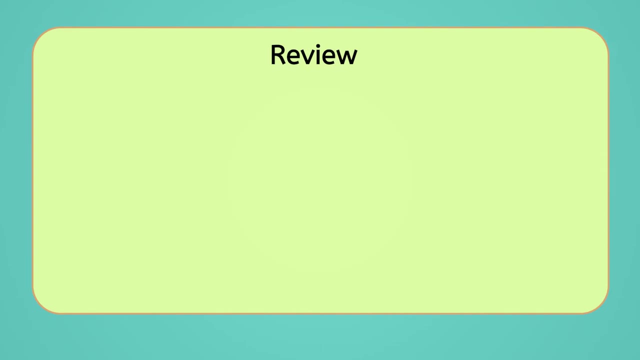 So we've tied it to the bucket, We pull down on the rope which turns the wheel, lifting the load, And there we go. We've gotten the slime to the top of the stairs. While I finish setting up my prank, let's review everything we've learned today.